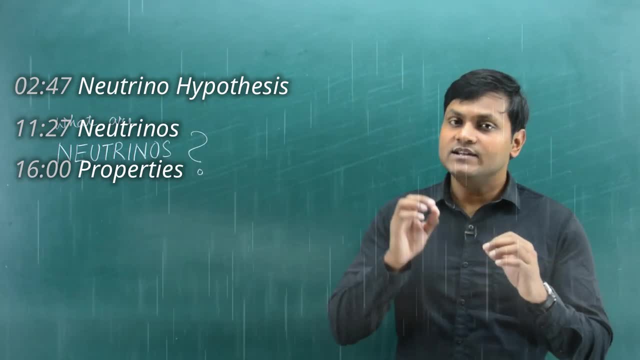 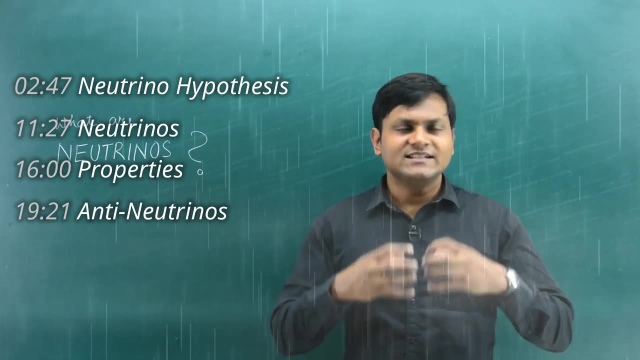 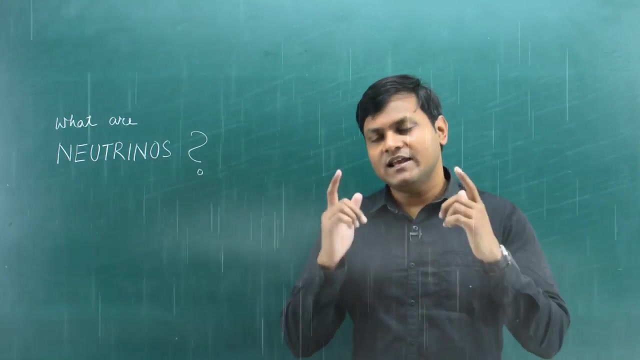 finish this video discussing a very important property that distinguishes neutrinos from anti-neutrinos, which challenged a very basic assumption of our universe and its physical laws, which has to do with what is known as parity symmetry. So, without wasting too much time, let's get straight into the 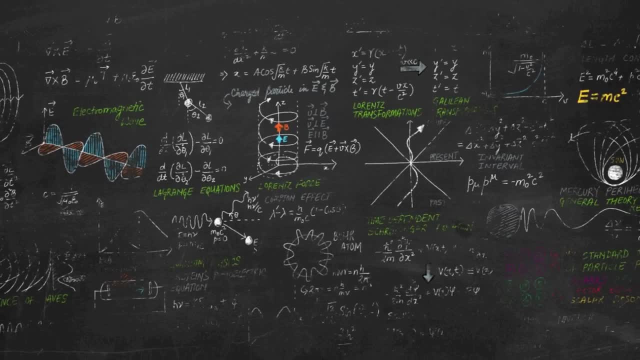 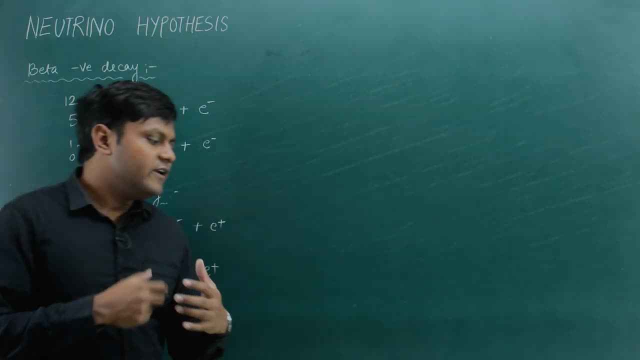 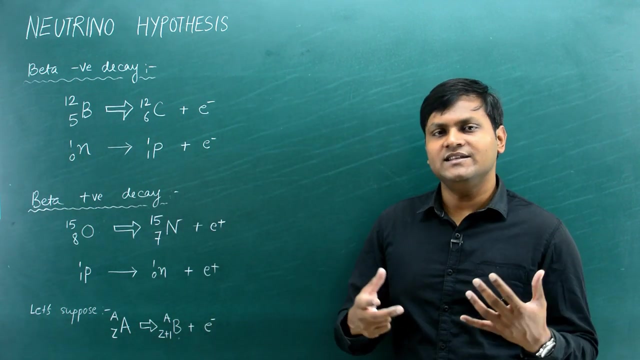 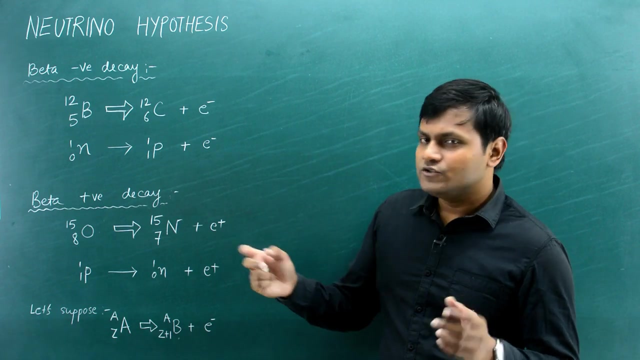 video. The very first time we even caught a hint that these kind of elusive particles even exist in nature is by the study of beta decay reactions. So I have a beta negative decay and beta positive decay. here I have two examples, So just a brief recap. In a beta negative decay I have the example of boron. 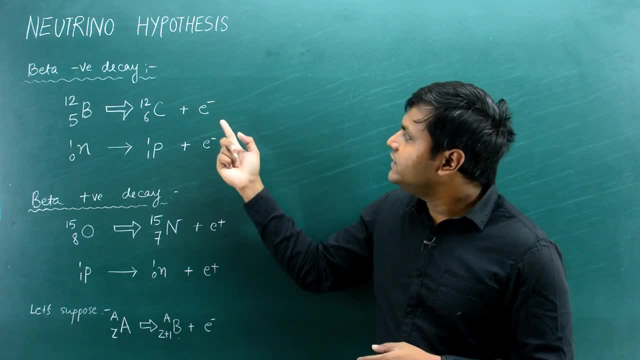 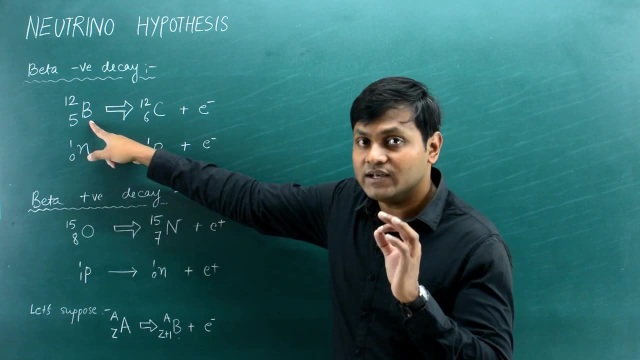 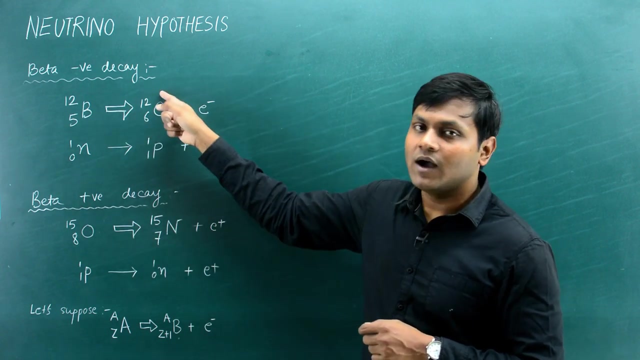 12,, which gets converted to a carbon 12, leads to the emission of an electron. What is happening is that the neutron particle inside the boron 12 nucleus spontaneously gets converted to a proton, thereby increasing the atomic number, transforming the boron to a carbon and releases an electron. 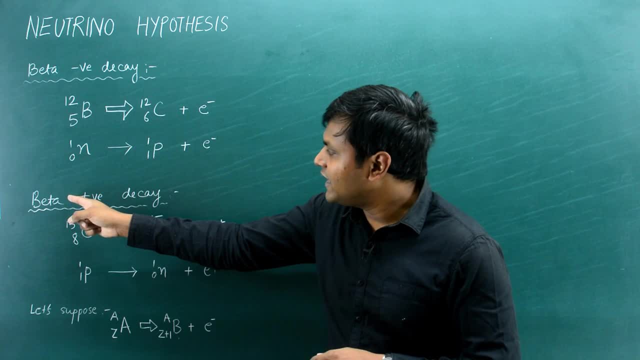 A very similar kind of a process also happens, which we know now as beta negative decay. So we have two examples. So just a brief recap: In a beta negative decay I have the example of boron 12, which gets converted to a carbon 12, releases an electron and releases an electron, A very similar kind of 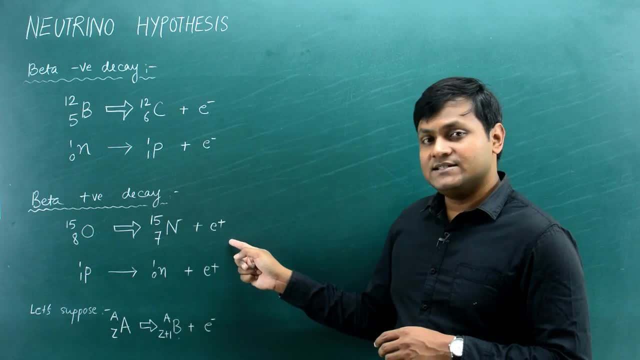 a process also happens which we know now as beta negative decay. So we have two examples. So just a brief recap. So here I have an oxygen 15s becoming a nitrogen 15s and leads to an anti-electron here in instead of a. neutron to proton to proton to neutron. transformation takes place where a proton inside the oxygen 15s spontaneouslyissely transforms into a neutron, does making the nucleus nitrogen, and leads to the emission of an anti electron. Other kinds of beta decay reactions are also there. You have electron. 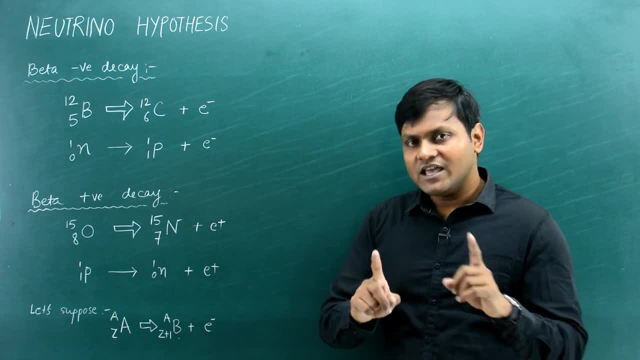 capture, you have inverse beta decay reactions. However, for the sake of discussion, I'm only going to consider one type of Leo 배 계산수, which components are the beta positive decay reactions. the beta positive decay reactions are the beta negative decay reactions. However, for the sake of discussion, I'm only going to consider one type of beta organic decay reactions. 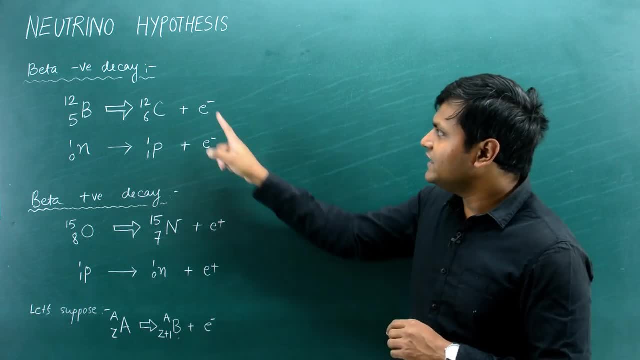 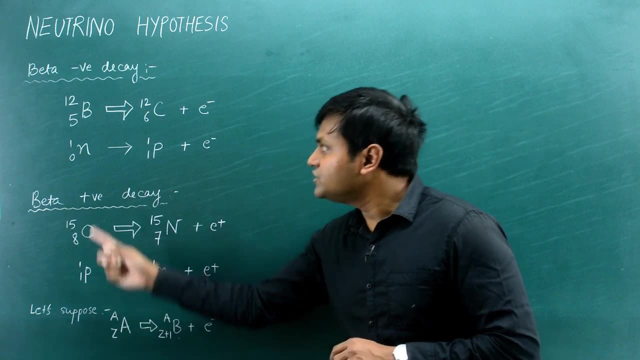 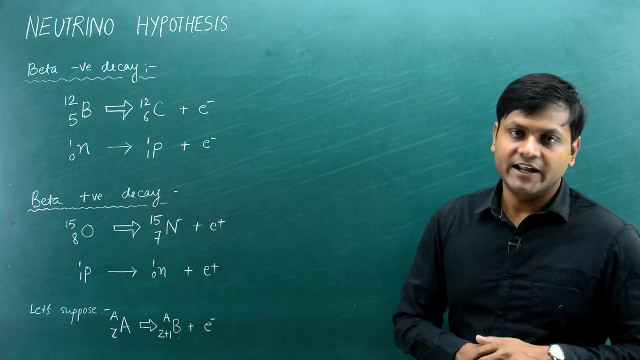 one type of a decay process. let's take the negative beta decay process. so in the general negative beta decay process you have a particular elemental nuclei inside which the neutron gets converted to a proton, so the atomic number of the nucleus increases, the elemental structure changes leads to the emission of electron. a study of these kinds of negative beta decay reactions: 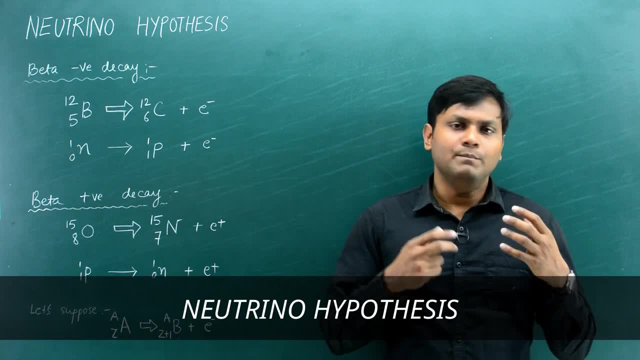 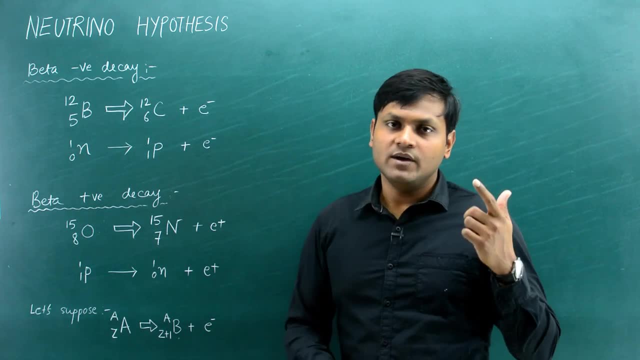 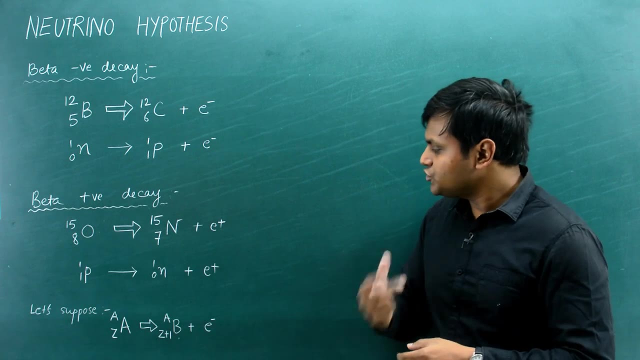 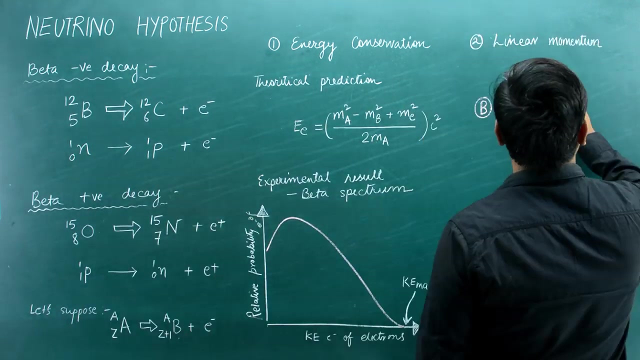 came up with some very bizarre conclusions- all right conclusions- regarding energy conservation, momentum conservation and angular momentum conservation. so let's look at a few theoretical predictions as well as some experimental data associated with the negative beta decay process. so, if you look at this particular reaction, a very general negative beta decay process, 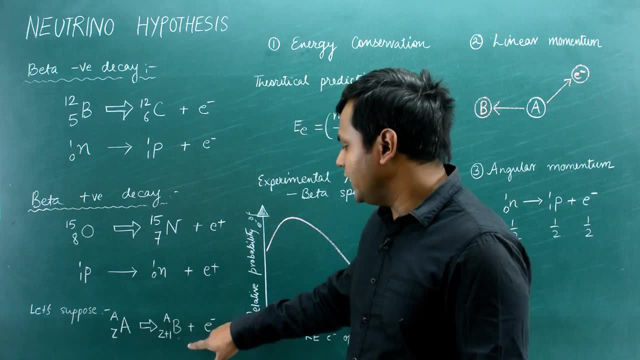 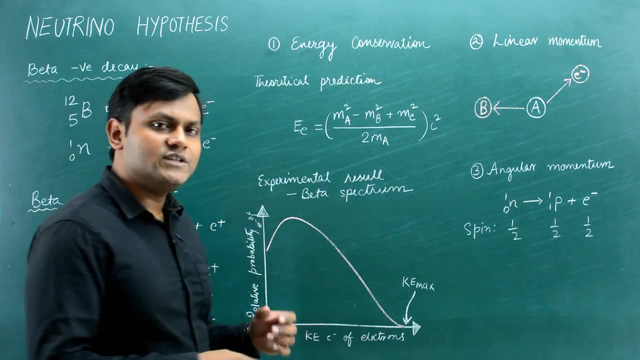 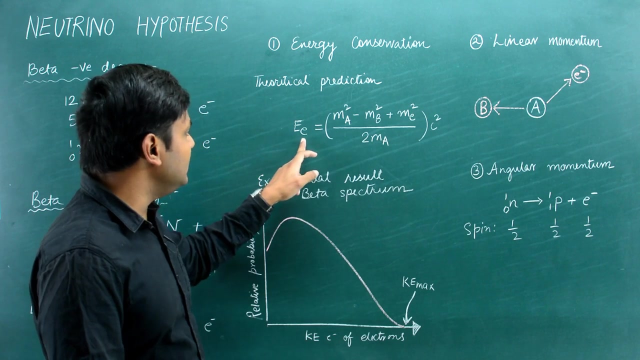 so if you look at this particular reaction, a very general negative beta decay process where A nuclei becomes converted to B nuclei and releases an electron- Now if you calculate the energies theoretically, then theoretically the amount of energy that the electron must carry off in this kind of a process is given by this expression where capital E, small e. this is 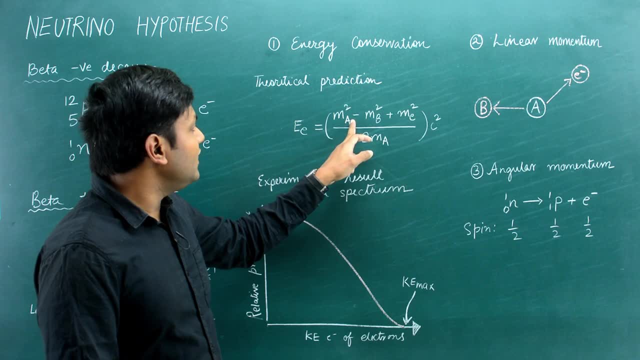 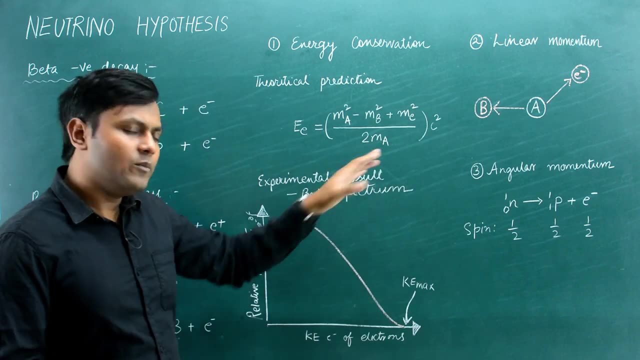 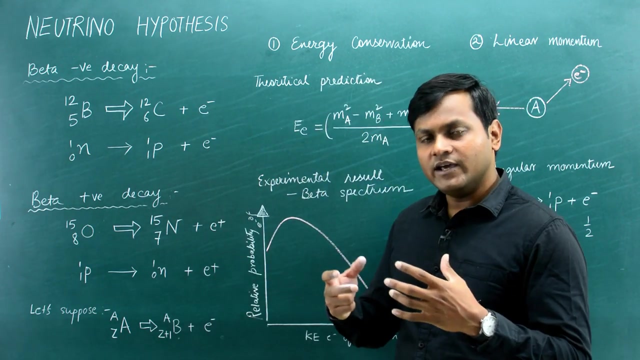 energy of the electron is equal to m a square minus m b square plus m e square, divided by twice m a whole multiplied by c square. Now how I obtained this? you can obtain this by looking at energy conservation, momentum conservation. The details of the calculation is not important here. 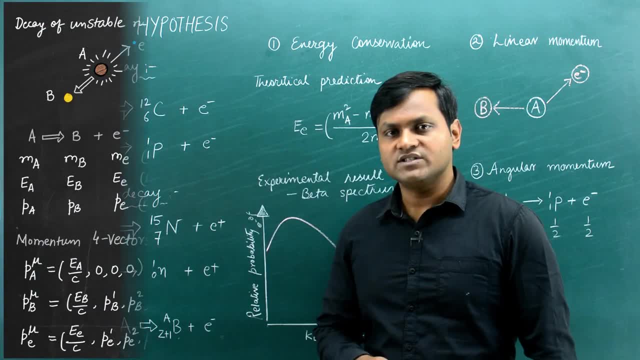 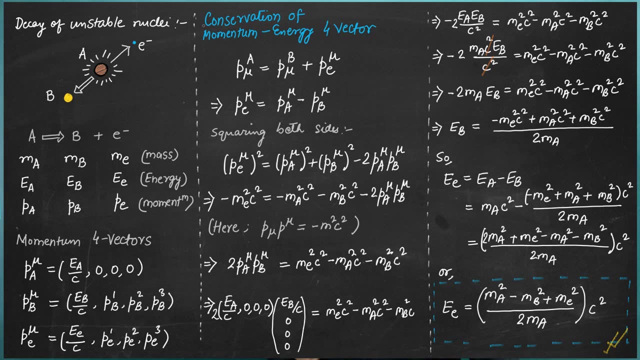 but if you are interested then I'll put up my calculations on the screen. You can pause the video and look at the exact calculation. I have used the conservation of four momentum energy vector to find out what should be the theoretical energy of an electron which is emitted while the 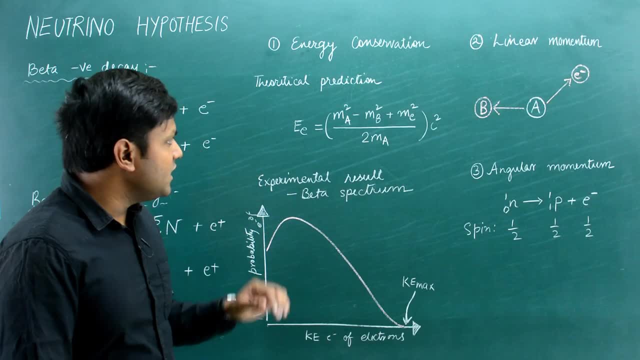 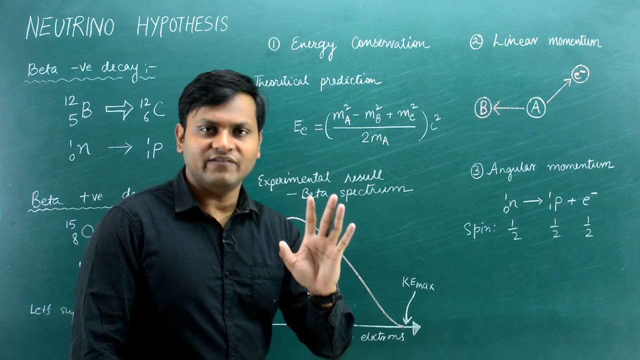 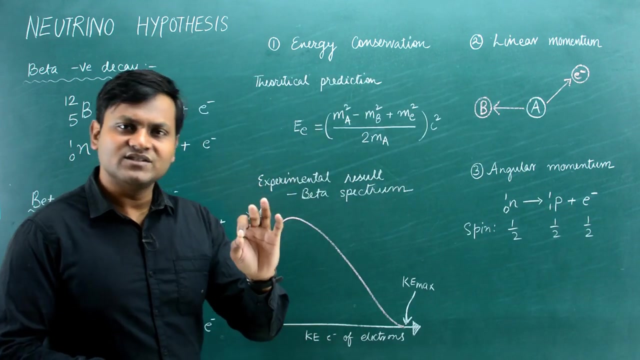 decay of an unstable atomic nuclei A takes place. Now, this is a theoretical prediction for the discussion. What is important is that this theoretical prediction is a constant value, constant for a specific reaction. If you have a specific decay process, then the energy of the electron must be a constant. It can only depend. 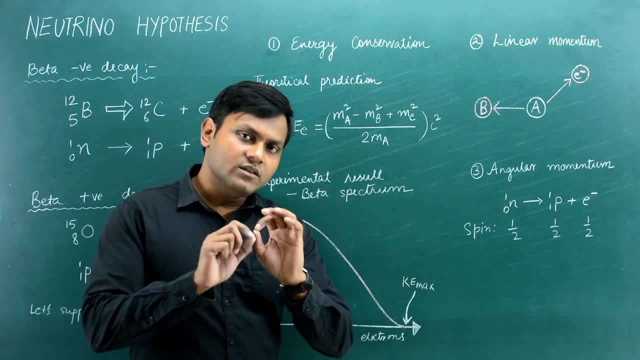 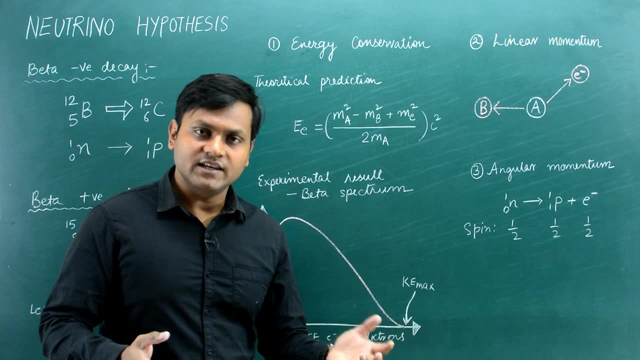 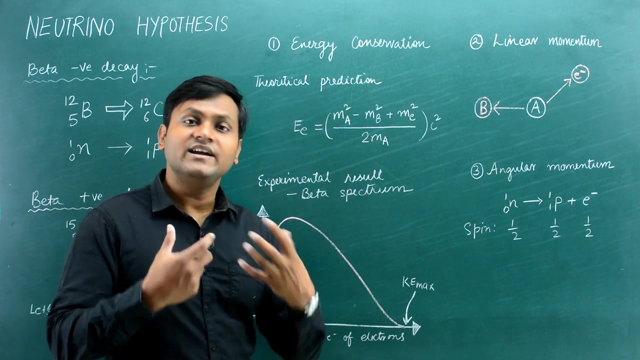 upon the masses involved and the speed of light. All right, this is a theoretical predictions. However, when experiments were done in various decay processes associated with the beta decay for different different reactions, it was found that the energy of the electron must be constant. So the energy which is emitted during this kind of a reaction, or the kinetic energy of the electron, 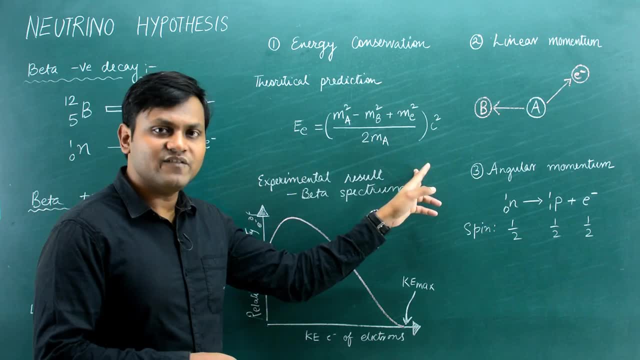 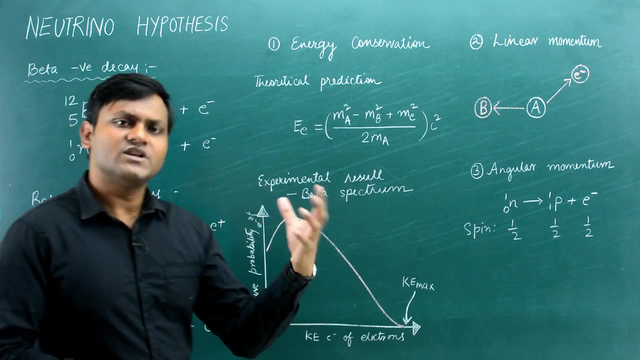 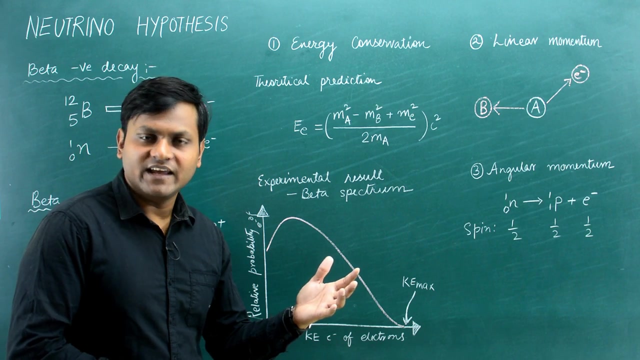 which is emitted during these reactions did not have a fixed value, but rather it formed a continuous distribution. All right. so a number of studies of this kind of a beta decay process found out that the energy of the electron emitted in any one given experimental decay reaction fell into a 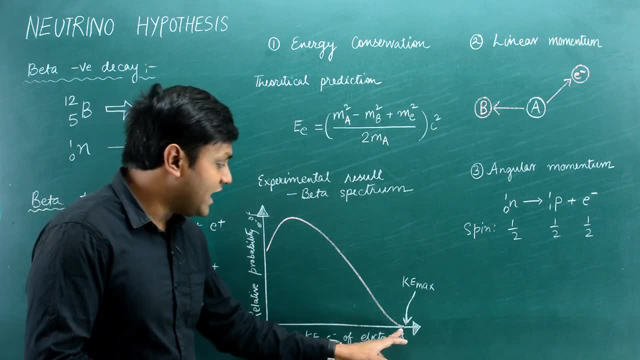 spectrum. That means it could have very low values. it could have a higher value, which has an upper limit, and it could be somewhere in the middle of the spectrum. So in this case it could have a very high value, which has a very high upper limit, and it could be somewhere in the middle of the spectrum. So 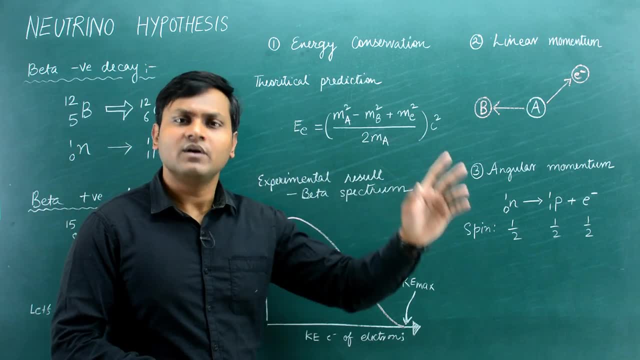 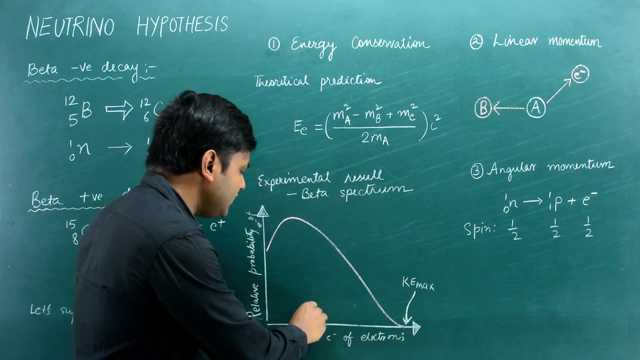 middle, when one particular decay process is studied many number of times and the energy of the electron is calculated. the electron may have energy somewhere. here. it may have an energy here. it may have an energy here, it may have an energy here. but if you plot the number of electrons, 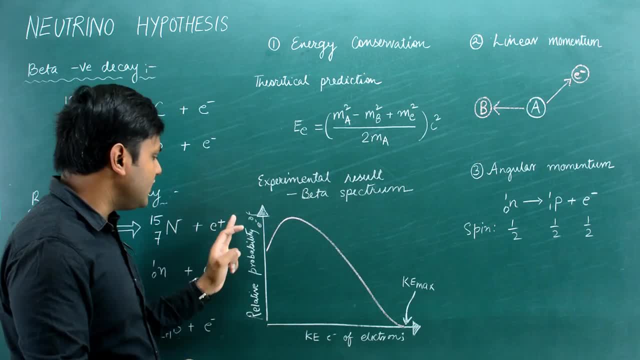 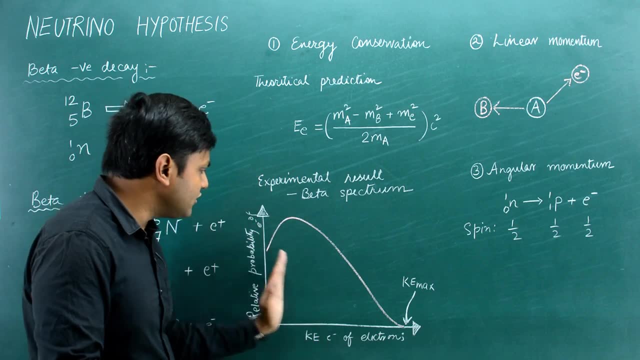 having the energies in a given range, then the y-axis here represents the frequency or the relative probability of the electrons, and the x-axis here represents the kinetic energy. so vast majority of electrons will be somewhere here and as you go higher up the number of electrons will decrease. 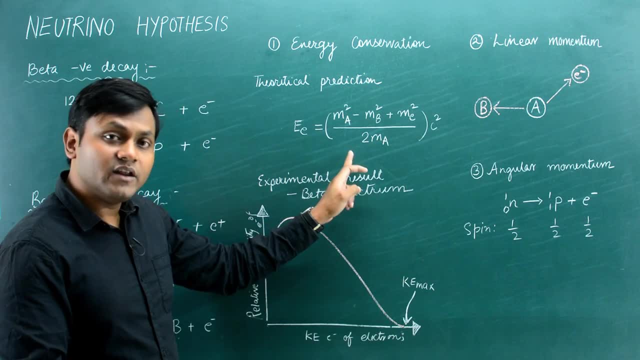 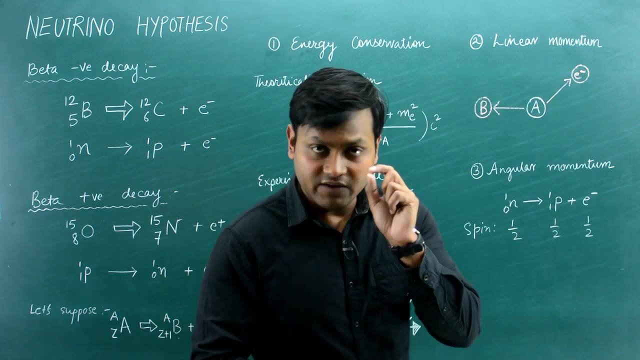 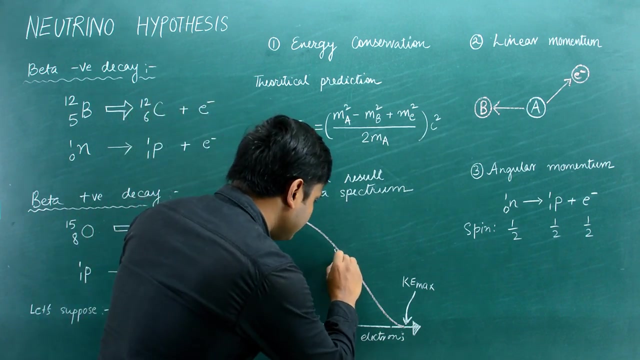 in fact, this upper limit represents our theoretically calculated value. now, how is it possible that theoretically we are getting some kind of an expression which has giving us a fixed value which is supposed to be here, but experimentally the electron turns out to be, let's suppose, somewhere here. all right, if the electron turns out to be here in a given reaction, then that means 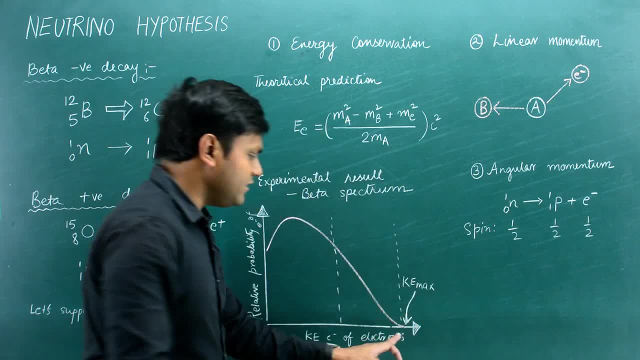 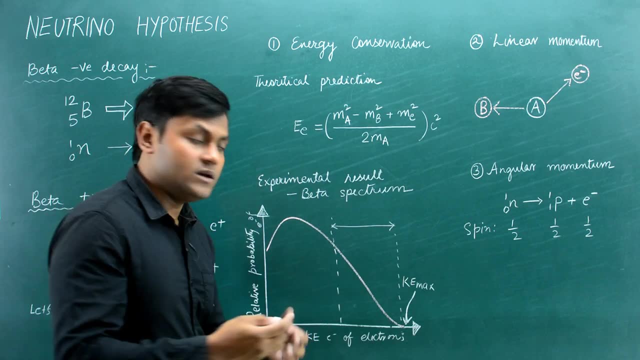 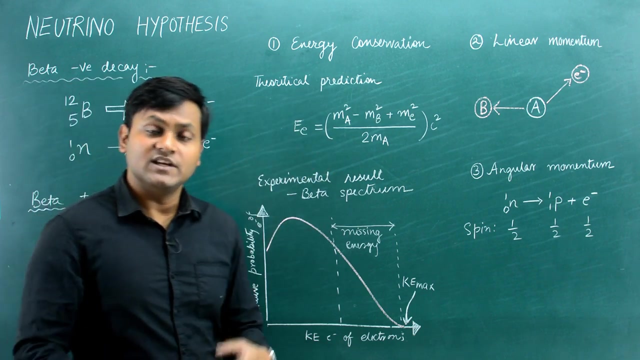 there is a discrepancy between the expected result and the actual obtained result. so a huge amount of this energy was not explained. you can call this the missing energy. so there was an amount of energy which was not explained by theoretical predictions. in fact, it looked as if the conservation law of energy 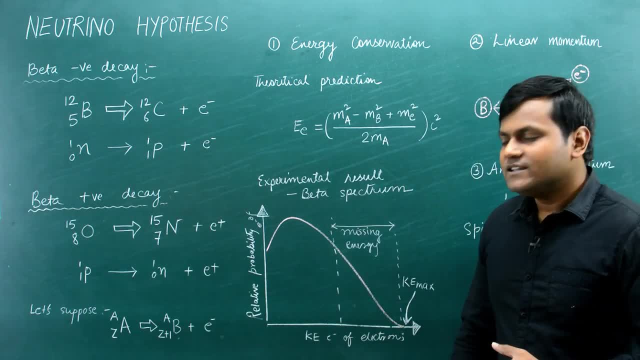 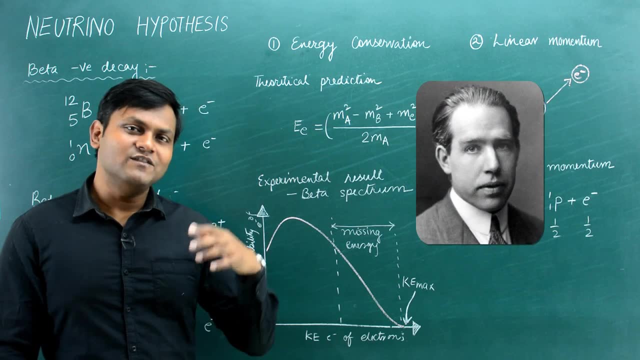 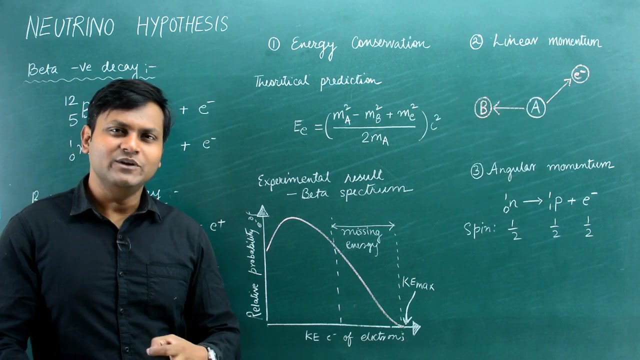 itself is being violated in this kind of a process. this was such a big challenge at that point of time that one of the great physicists, Niels Bohr, who gave the Bohr's law of conservation. he even said that maybe energy conservation law is not true and we need to get rid of that principle. 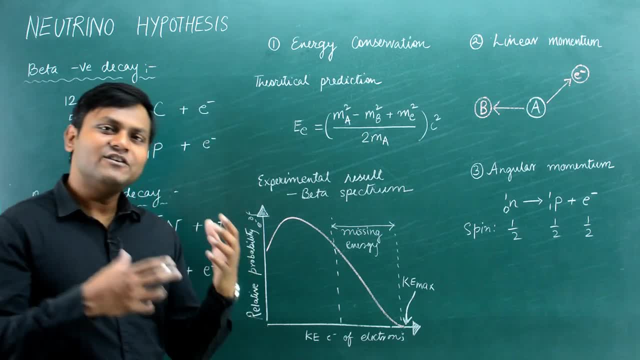 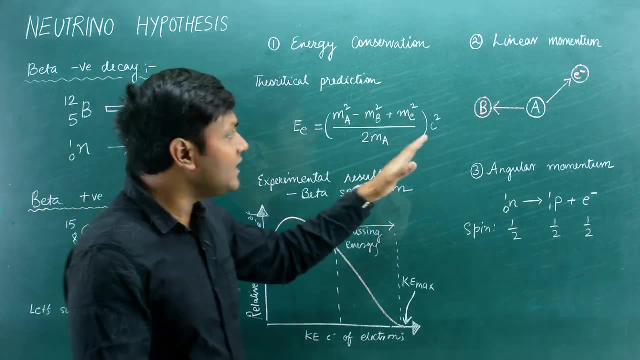 such was the state of physics at that point in time. and even worse, not just energy conservation, even other laws were being violated: the conservation of linear and angular momentum. so if you look at the emission of the electron once the decay takes place and the recoil of the daughter nuclei, their 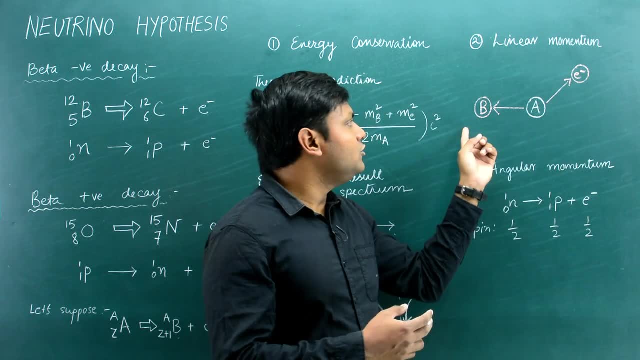 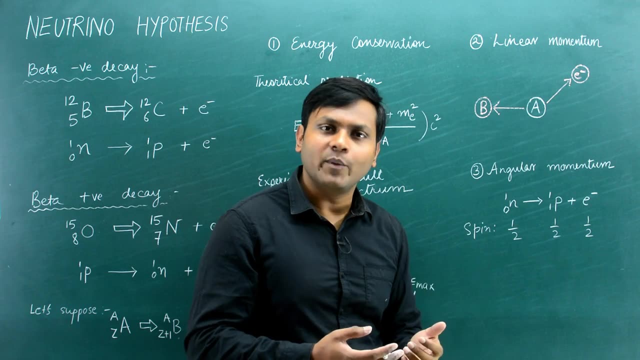 recoil directions were not opposite. they had a non-opposite directions. this means that they this kind of a process where their directions are not opposite will not conserve linear momentum right. so in a way, this kind of a beta decay process was also violating conservation of linear momentum. 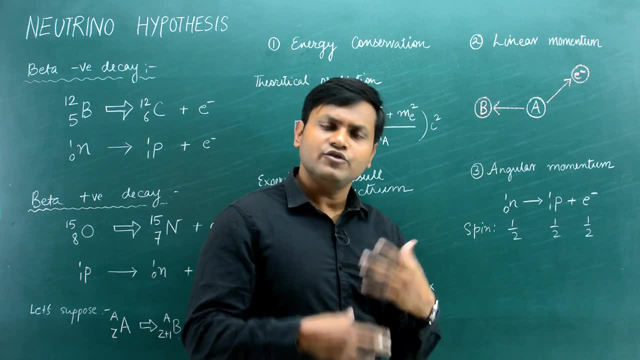 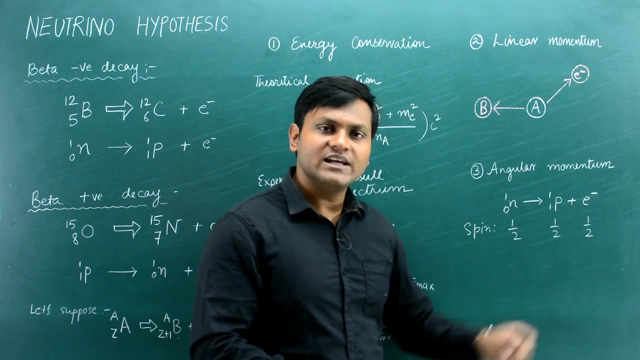 principle and even if you look at the concept of angular momentum, it was also violating the concept of angular momentum principle. because if you look at a neutron converting to a proton and an electron, neutrons, protons and electrons are fermions. that means they have spin. half, all right, half, half half. 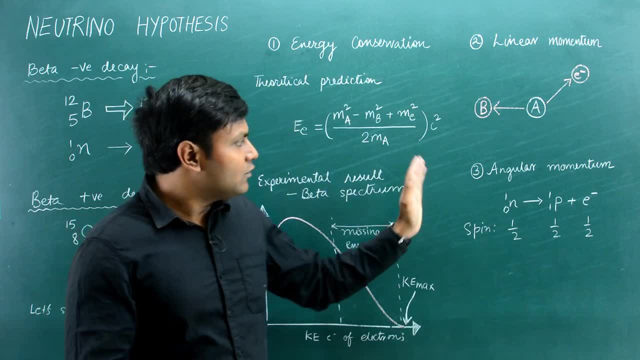 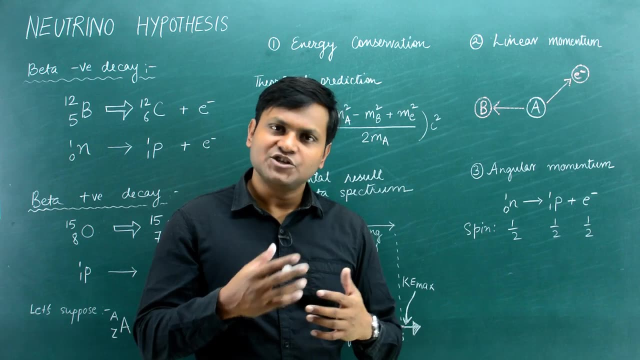 this kind of a process is not possible now. usually calculation of angular momentum is quite a complicated process and it is not possible to calculate the angular momentum principle because quantum mechanics puts up lots of restrictions in the nature of these kind of a calculation and also the idea of a spin is very different from classical spin. i guess you know all. 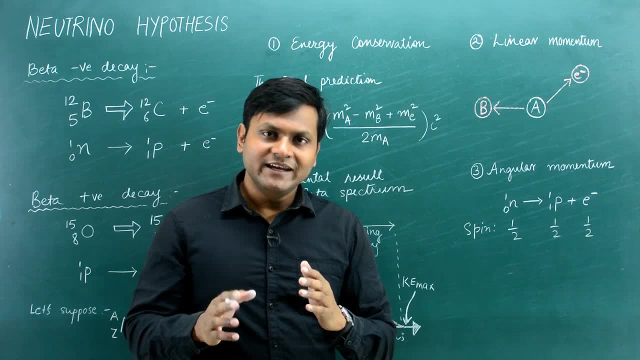 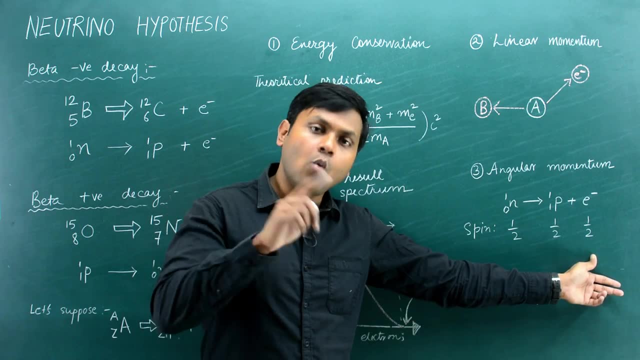 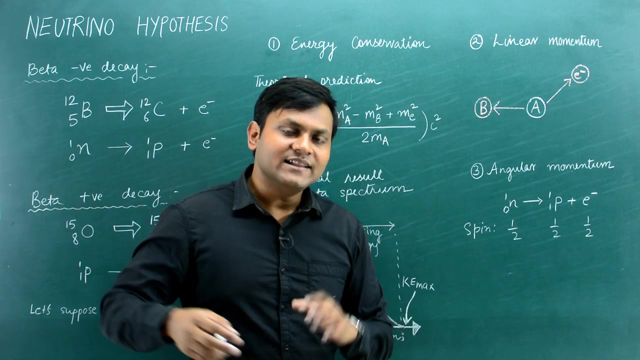 of those things, but without going too much into details. there are few rules that are associated with the quantum number, so half here represents this spin quantum number associated with these elementary particles. but from this quantum number you can find out the actual angular momentum and there are certain rules associated with the angular momentum and the quantum momentum. 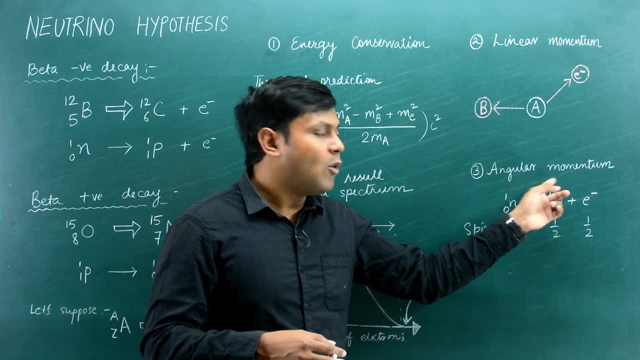 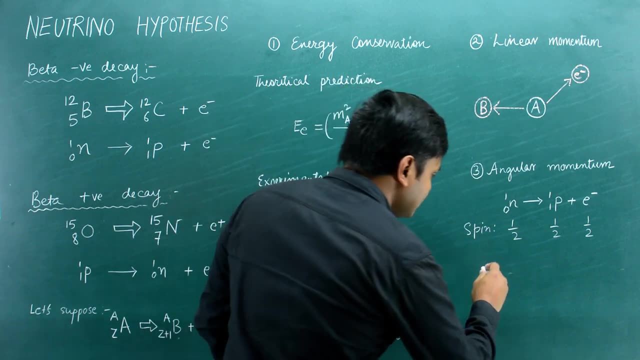 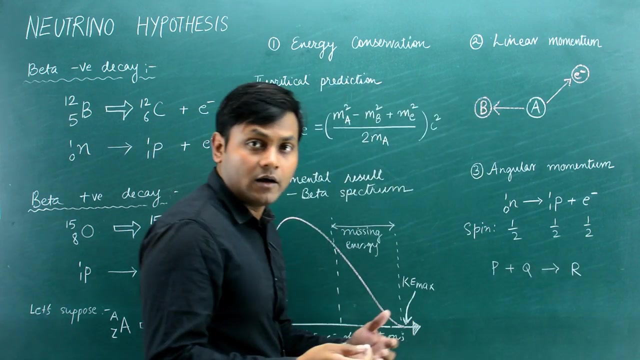 this kind of a quantum number. otherwise the angular momentum associated with these kind of a quantum numbers will not be conserved. So for example, if I take a very generic example, let's suppose some kind of an elementary particle P and another elementary particle Q becomes another elementary particle R. Now I'll just give you a little bit of a taste of what kind 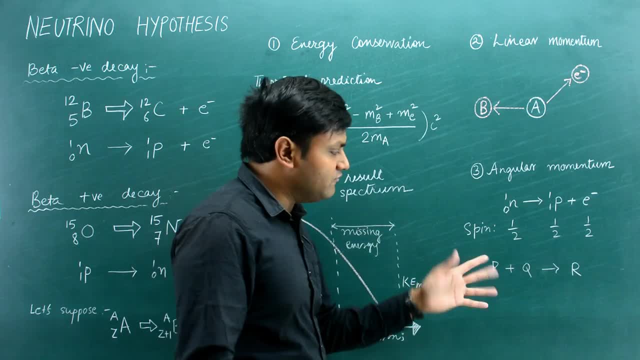 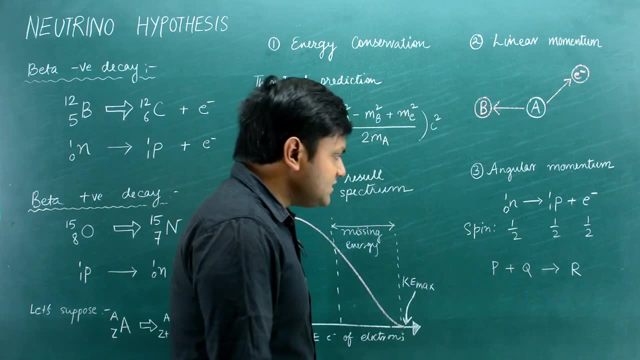 of spin, quantum number values are possible and how they are involved in a given reaction. So the rules of conservation of angular momentum, tells us, is that if P, Q and R are some elementary particles, and let's suppose P and Q has angular momentum of, let's suppose, some integral multiple, 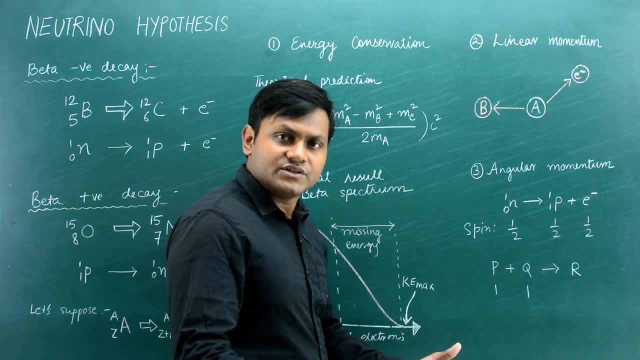 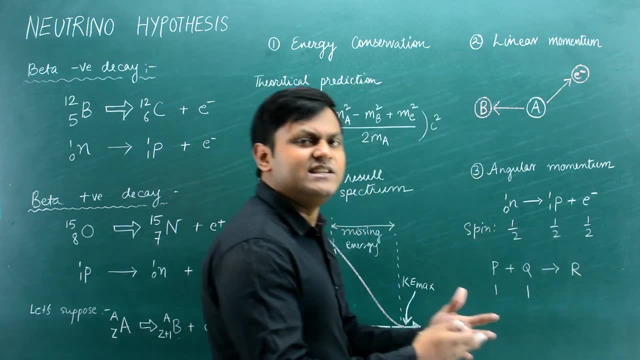 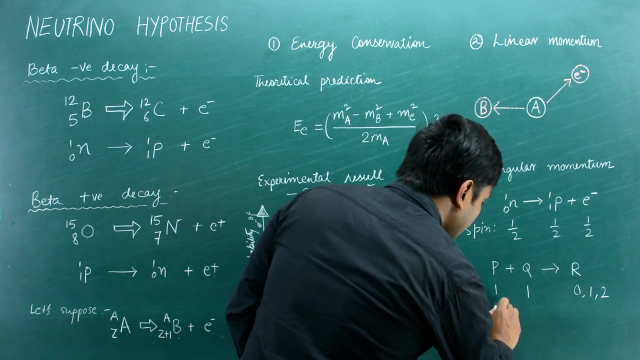 of h cross or a spin quantum number of integers, then the rules of angular momentum tells us that the final product must also have some kind of an integer spin quantum number, like maybe 0,, maybe 1,, maybe 2.. If P and Q has spin quantum numbers of half and half, let's suppose 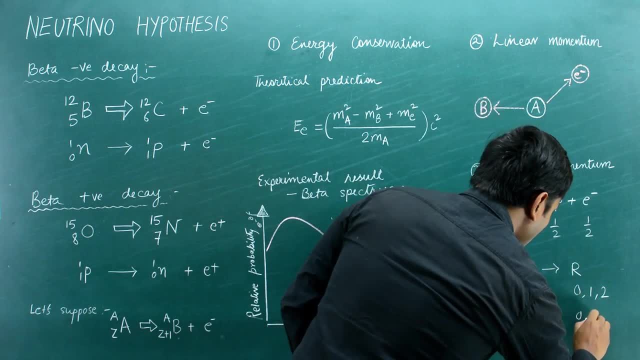 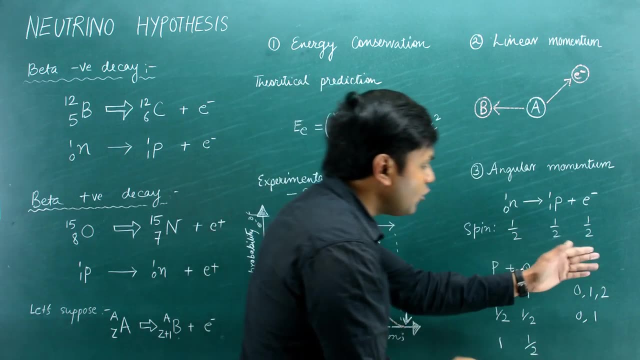 then the final product will have spin quantum numbers of 0 and 1. that is basically an integer. If P and Q has spin quantum numbers of 1 and half, then the final product, R, will have spin quantum numbers of half or 3 by 2.. So these are some of the few rules associated with. 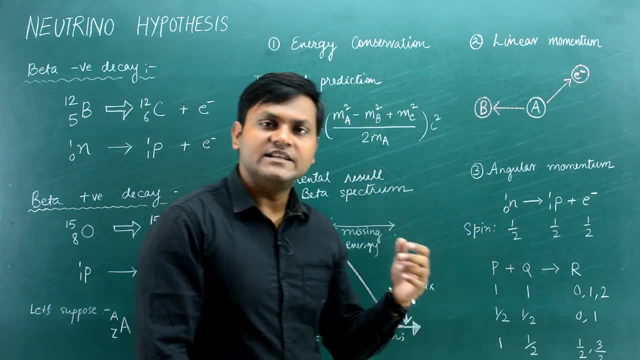 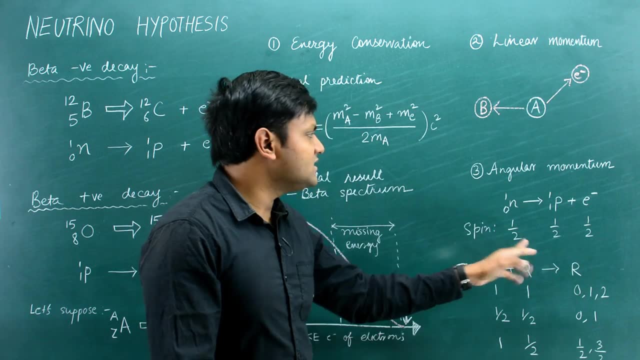 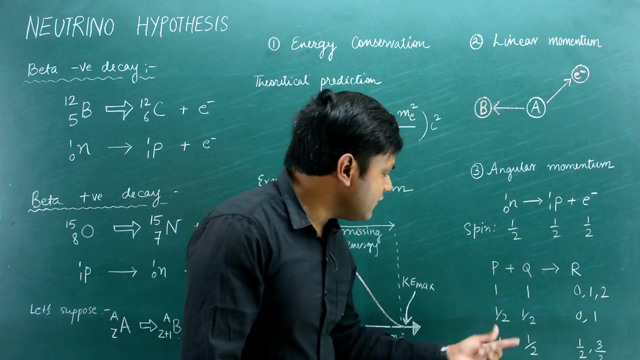 how spin quantum numbers are associated with the decay process in elementary particle physics. Now, based on these rules, it can be seen that in this particular reaction the conservation of angular momentum is being violated. On one side you have half and half. on the other side you have half, which is not allowed. 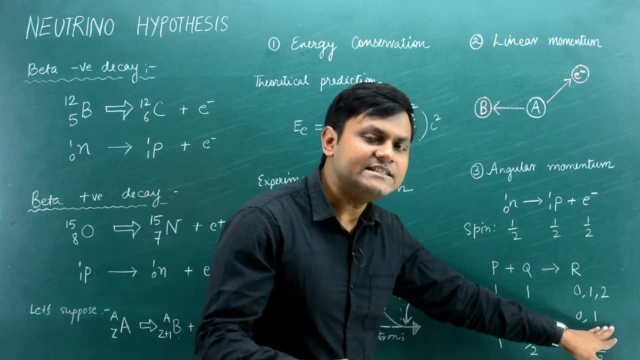 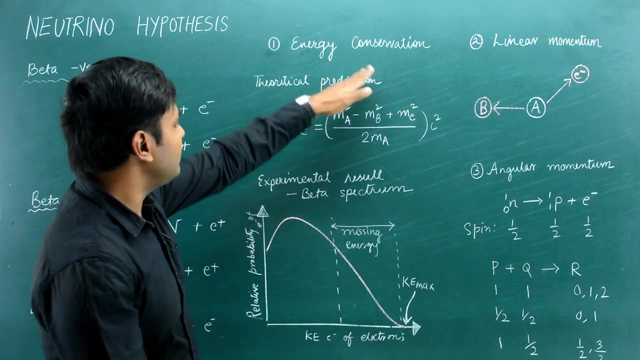 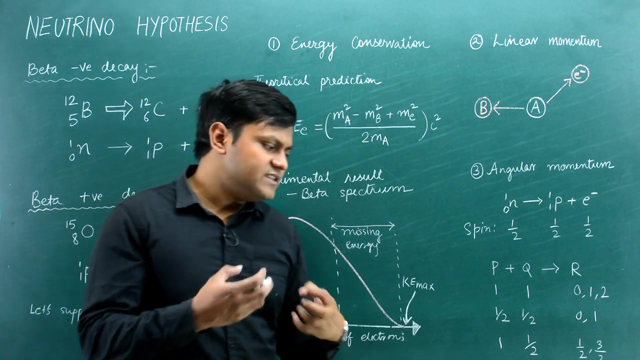 If you have half and half on one side, you should have 0 or 1 an integer on the other side. but that is not happening here. So these violations of the conservation of energy principle, the conservation of linear momentum and the conservation of angular momentum was kind of a very difficult time for physics. 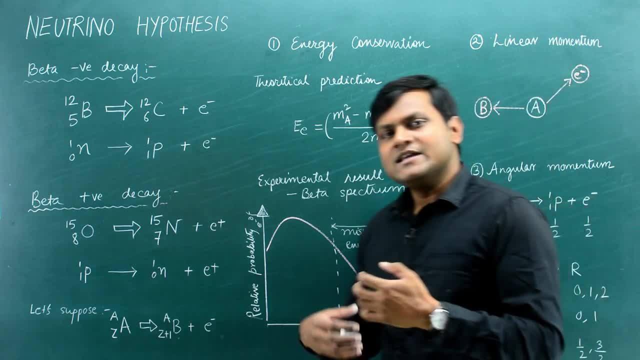 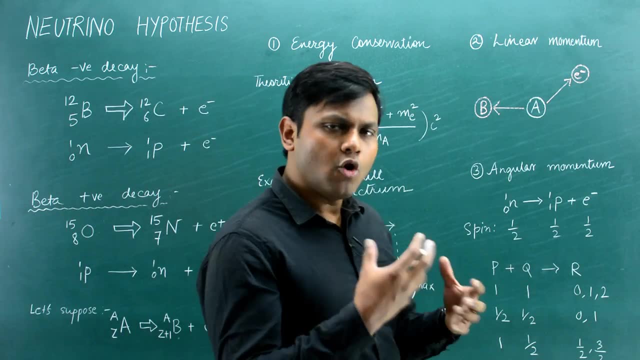 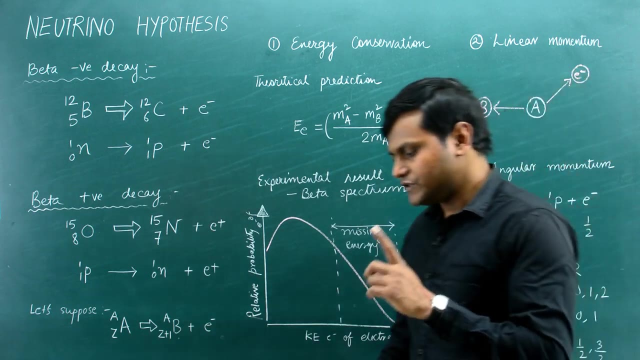 because these are some of the fundamental conservation laws in physics. So the beta decay processes created a lot of trouble at that particular point in time because they somehow seemed not to follow the known conservation laws. Now, at that point in time, a scientist by the name of Wolfgang Pauli, you must have heard- 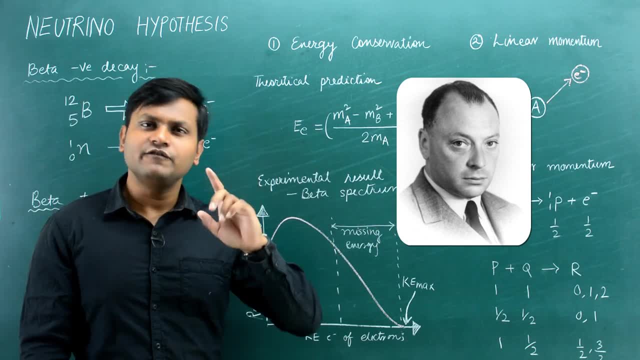 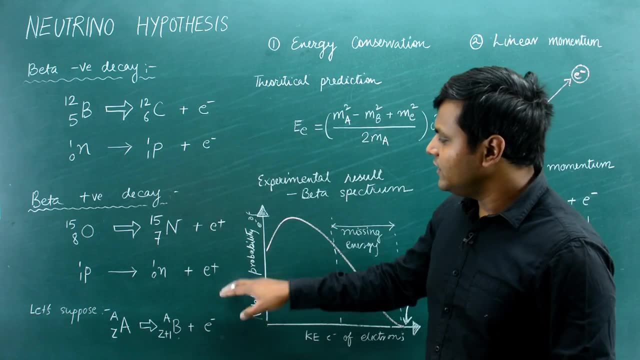 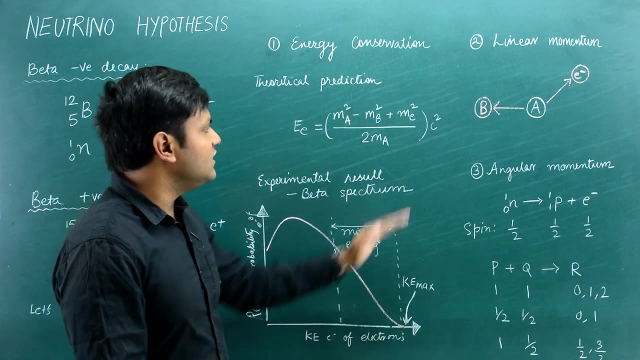 of him. he gave the Pauli's exclusion principle. he suggested for the first time that in this kind of a decay process, if we include another particle, if we say that another particle is involved in the decay process, then we may be able to save the violation of these three. 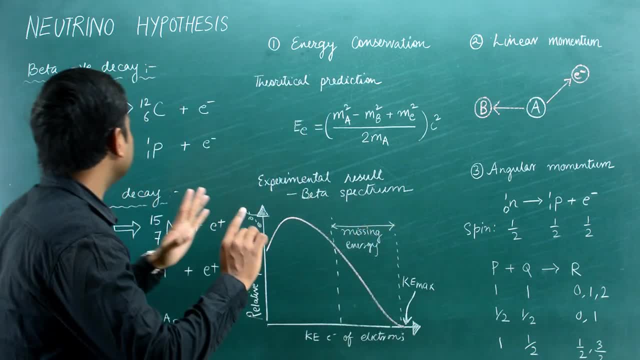 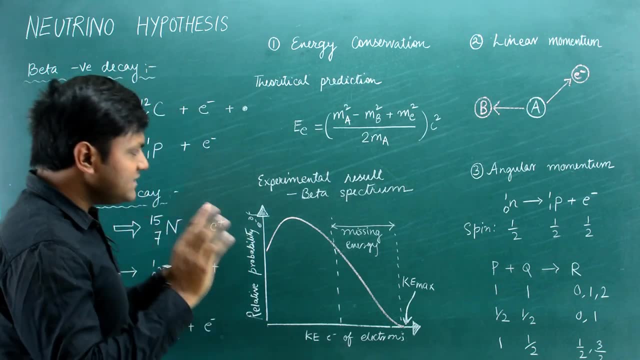 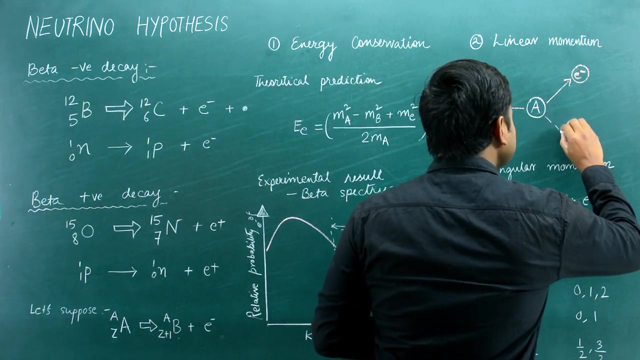 fundamental conservation principles. So let's suppose that in this reaction another particle is also emitted. All right, if another particle is emitted, then we may say that that particle carries of this missing energy, then that particle conserves linear momentum for this kind of a three-body decay process and that particle might also lead to the conservation of angular 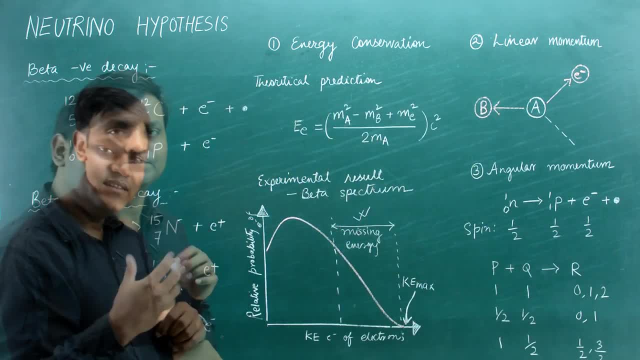 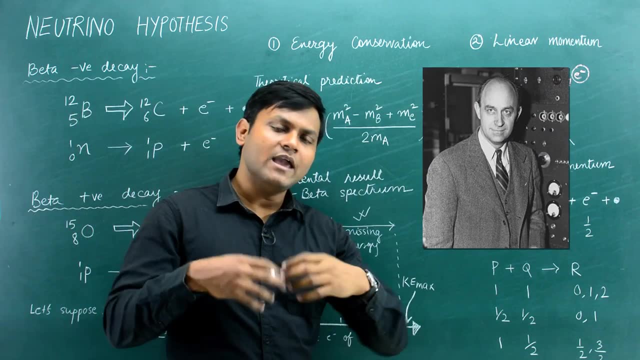 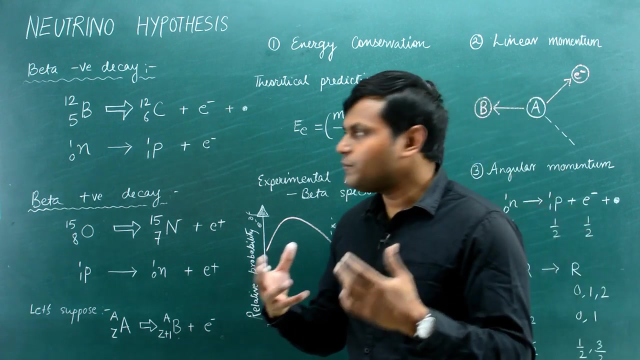 momentum, spin, angular momentum. This idea that was proposed by Wolfgang Pauli was later on taken seriously by Enrico Fermi, who came up with a theoretical foundation of beta decay processes, in which he used this idea to predict the existence of a particle by the name of neutrino. 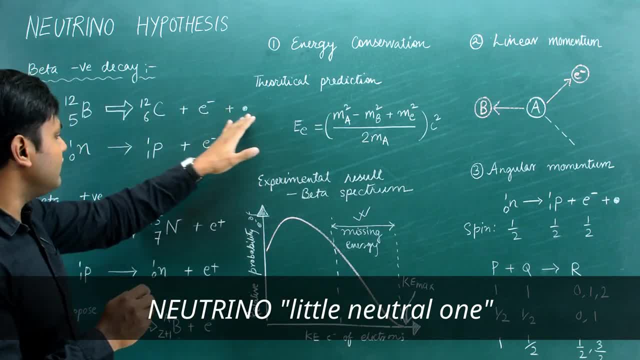 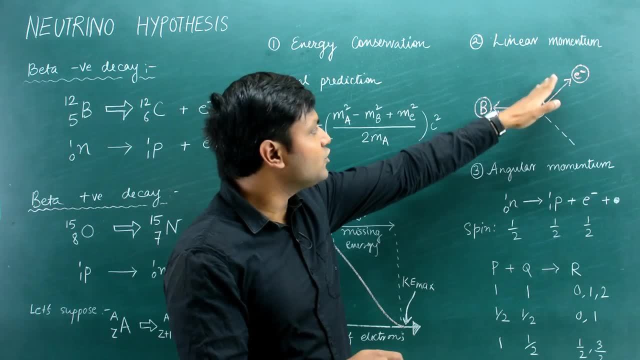 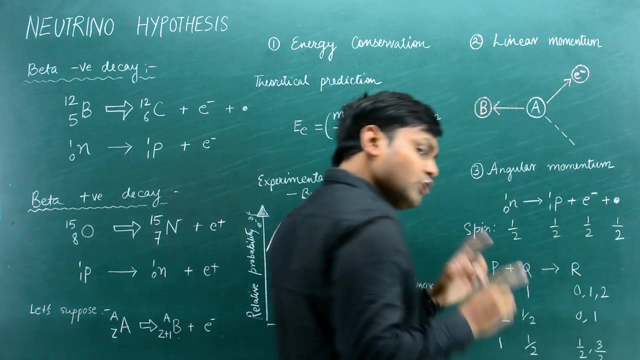 If there is a neutrino which is being emitted in this kind of a processes, then we can say that that particle is taking up the missing energy, that particle is also conserving the linear momentum and that particle must also have some kind of a half spin, So in a way that particle 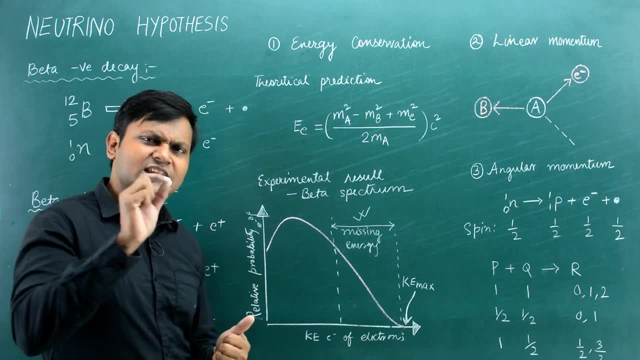 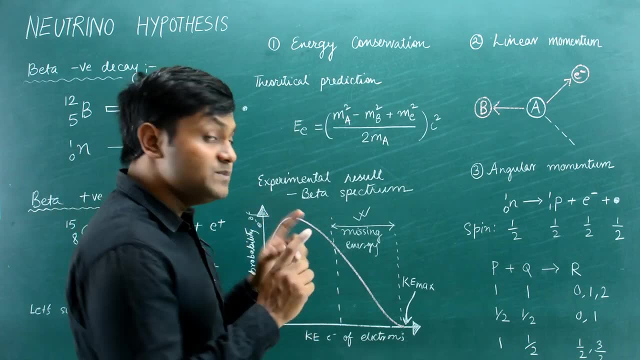 is a fermion. So, first of all, the particle must have very tiny mass, because it is taking energy from an electron. It must be very, very tiny. It must have very less mass. The particle must be uncharged. It must have zero charge, because why, If you look at this reaction, left hand side zero. 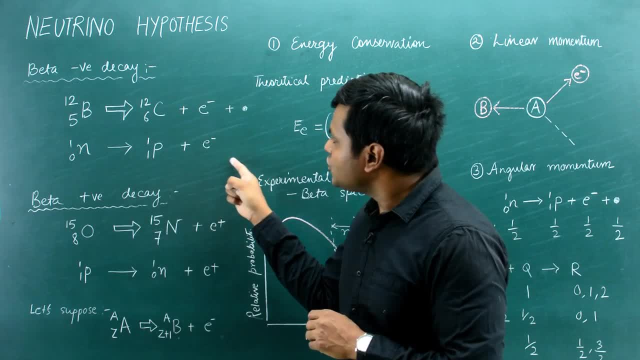 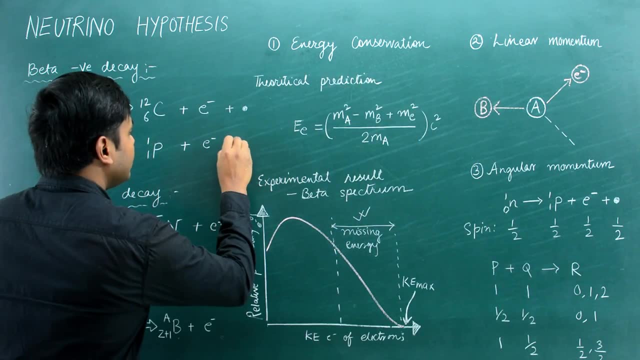 charge: right hand side: positive charge: electron has zero charge. So if you look at this reaction, right hand side negative charge. So charge is already conserved in this kind of a process, So the particle which is emitted must have zero charge. Alright, So the particle is emitted here. 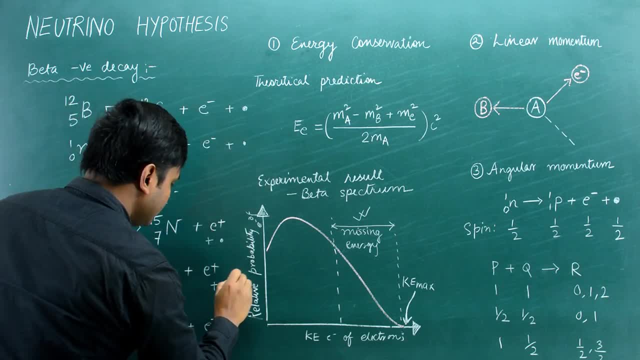 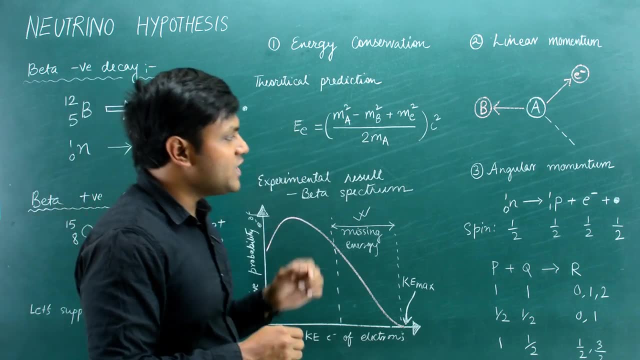 There might be a particle which is emitted here, There might be a particle which is emitted here and a particle which is emitted here. The particle must have extremely tiny mass, zero charge, and it must have half spin, because if there is a half spin, then this kind of a process. 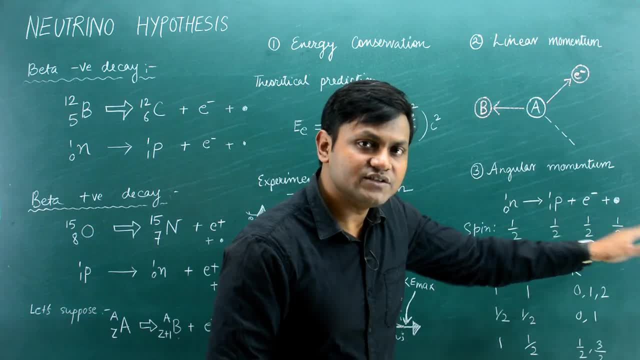 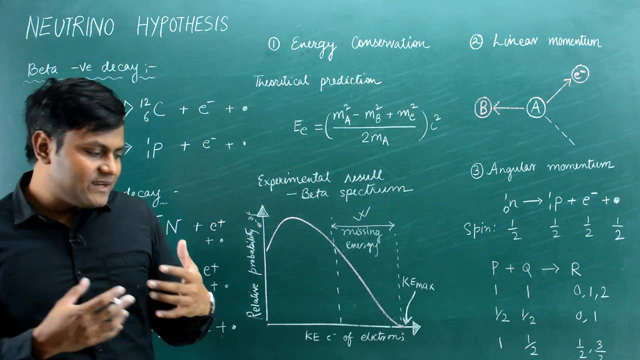 is balanced, because here you have three half integers. In that case the other side can have a half integer, So that particle must be a fermion, Alright. So such a particle was named as neutrino, or the little neutral one. Little means very tiny It. 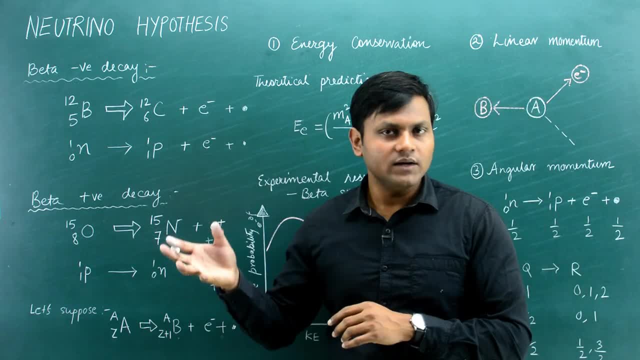 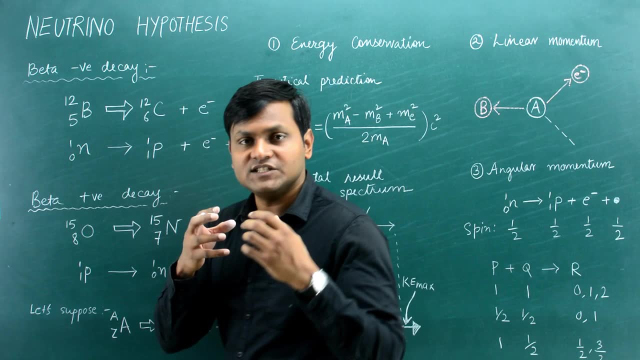 is named as little particle, as opposed to the neutron particle, which is quite massive Neutral one. it means it's uncharged fermion And later on, after a couple of decades, this particle was indeed experimentally verified to exist in nature. So, as it turns out, 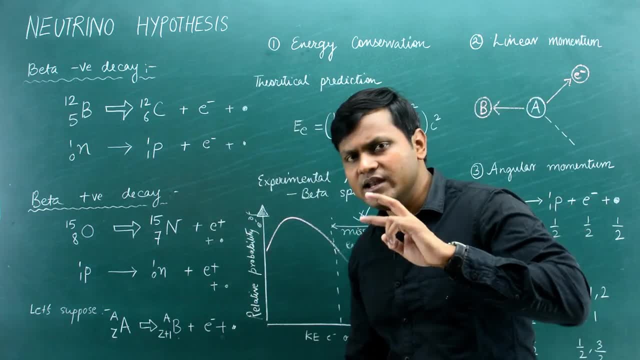 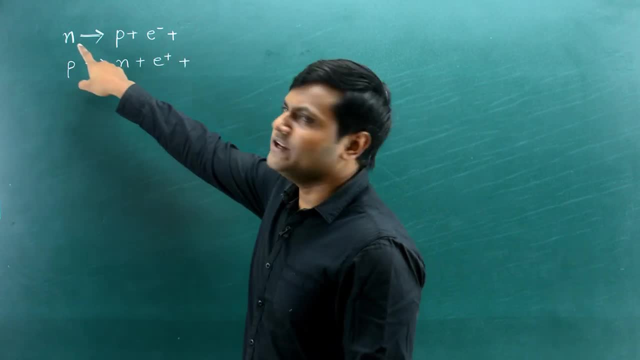 the particle emitted in negative beta decay and positive beta decay are a little bit different. So, as it turns out, the particle which is released in the negative decay process, when a neutron gets converted to a proton and also leads to the emission of an electron, is actually the anti.